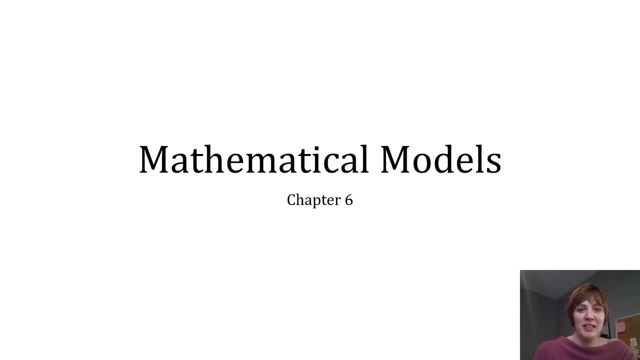 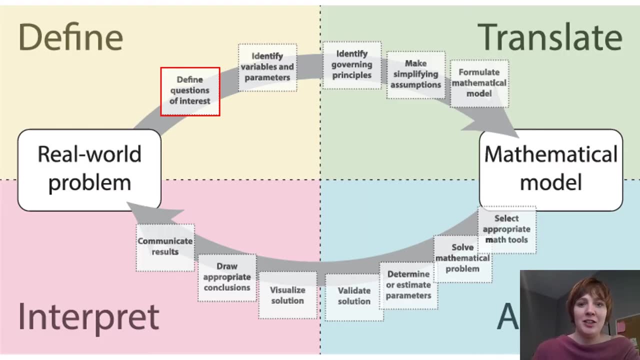 Hello and welcome to this mini lecture on mathematical models. To begin, we identify a real-world problem. This could be general, for example, how do fluids flow through the subsurface. or it could be more specific, for example, how long until contamination entering? 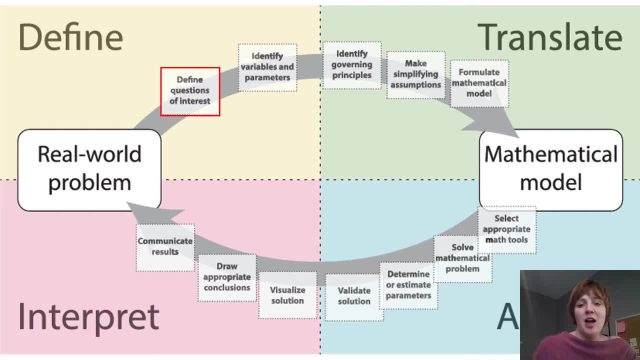 the ground at location X1 shows up in the aquifer located at X2.. Once we have defined our questions, we can begin to identify variables and parameters that will impact the behavior of the system. For example, we might need to know the flow rate. hydraulic conductivity. 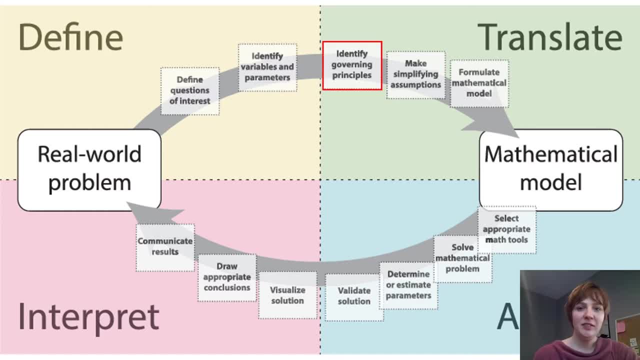 area, time, etc. As we start to build the mathematics that will enable us to answer our questions, we must begin with first principles to derive our governing equation. In hydrogeology we typically start with conservation of mass or energy, but math is not the answer. We 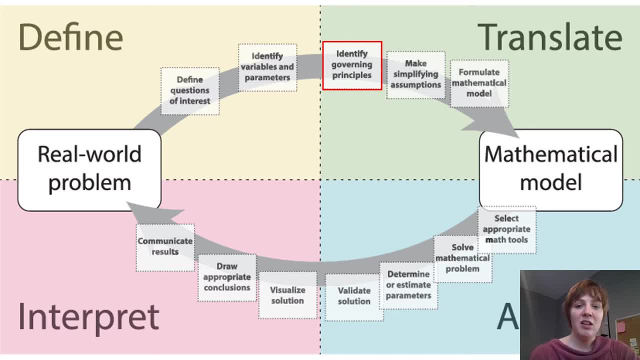 also utilize Darcy's law, the equation that states that discharge- the volume of fluid traversing a cross-sectional area per unit time is equal to the hydraulic conductivity of the material multiplied by the change in head across the volume of interest multiplied by the cross-sectional area of the discharge outlet. These derivations necessarily make 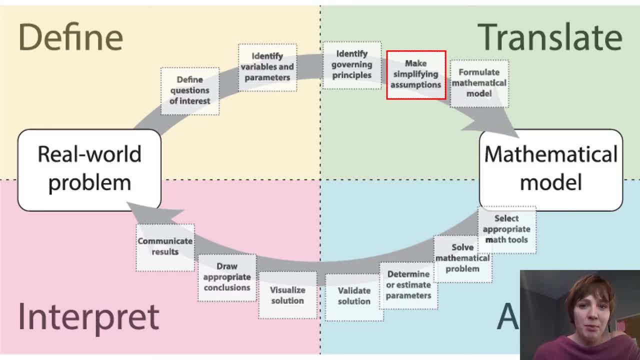 many simplifying assumptions. For example, if we want to know the volume of fluid that flows through the subsurface or the aquifer located at location X1,, we must first define the flow rate. For example, we might assume that flow is homogeneous, exotropic and steady. 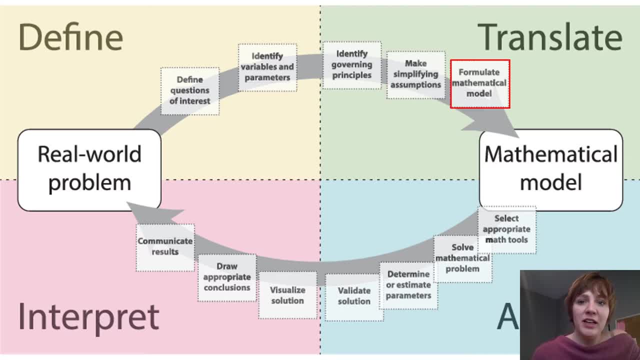 state. Once we have identified our general equations and made the appropriate assumptions about the system under study, we have formulated our mathematical model. The next step is to identify the appropriate tools that we need to solve the problem. That could be as simple as egoizing our calculator, or maybe Excel. 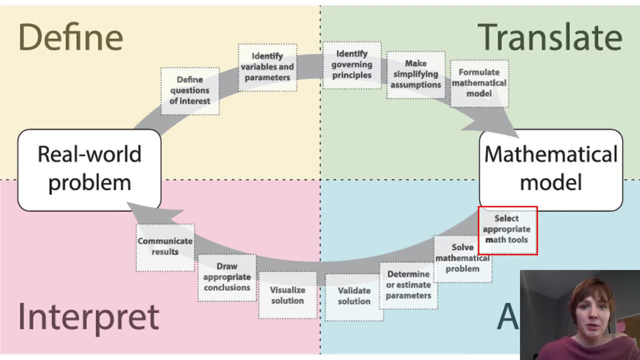 Once we have figured out what we need to execute the math, we can simply solve the problems. We plug our specific values into each of the parameters in the model and solve the model. This enables us to calculate the time that flow will take to reach a location, what the